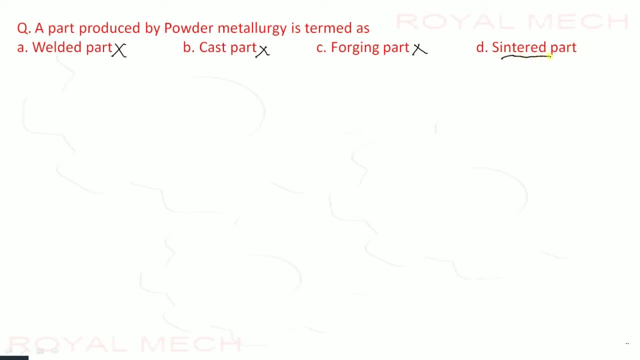 sintering part. So a part produced by powder metallurgy is called as sintering part. Which of the following method is used to make powder for brittle materials: Mechanical pulverization, Electrolysis, electrolytic process, Chemical reduction And automation? 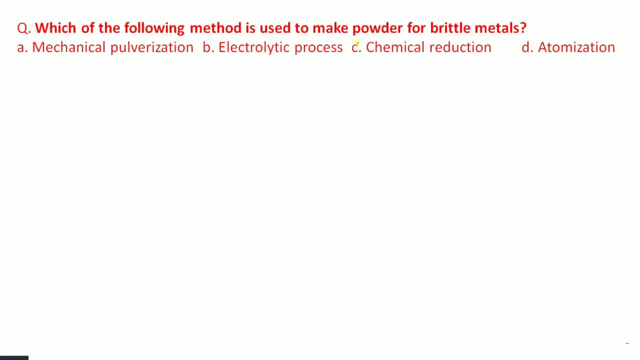 Mechanical pulverization, Electrolysis, electrolytic process, Chemical reduction and automation. Mechanical pulverization, Electrolysis, electrolytic process, Chemical reduction and automation. So the question is how the brittle material powder is made. So for brittle materials, mechanical pulverization method is followed. 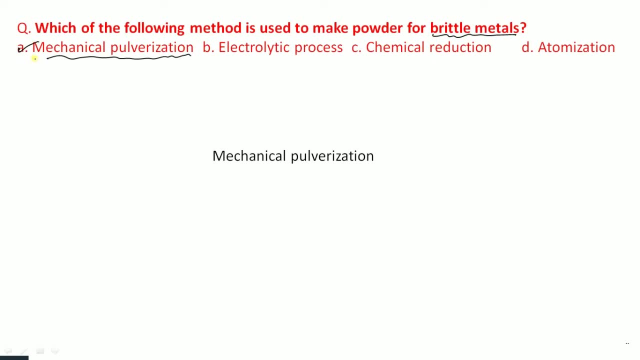 It is nothing but a grinding. So that is called mechanical pulverization. Which method is used to make powder of metals having low melting point? Mechanical pulverization, electrolytic process, chemical reduction and atomization. So to produce the powder of metals having low melting point, atomization is used. 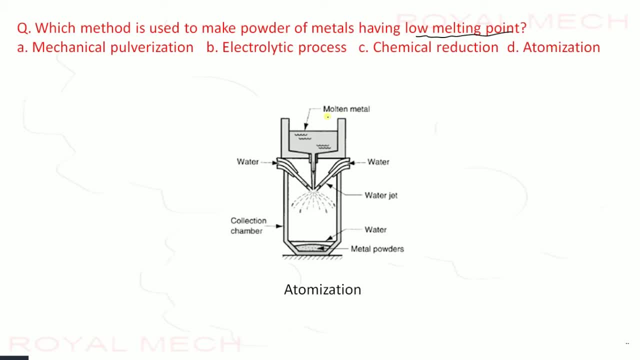 In atomization process. we can see in the picture molten metal. it is being poured and with the help of water jets the metal powder is produced. Therefore, option D is correct option to produce the powder of metals having low melting point. 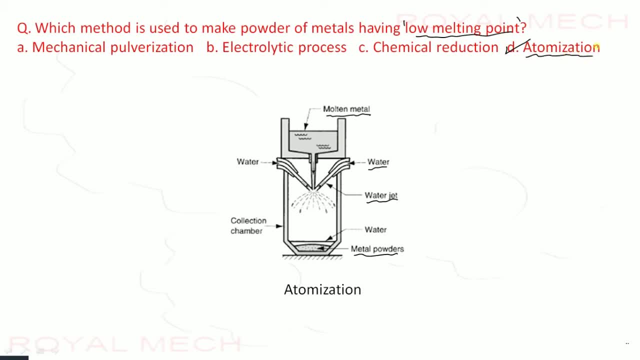 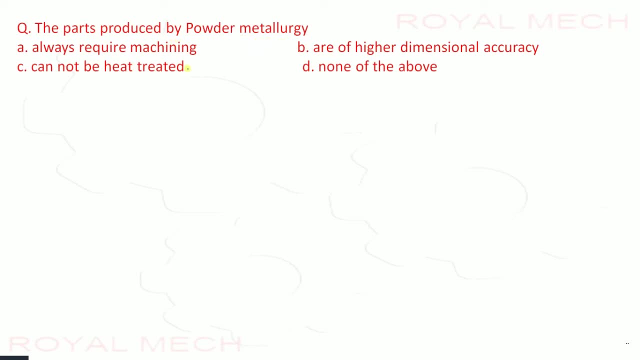 atomization process is used, So this is carried. The parts produced by powder metallurgy always require machining or of higher dimensional accuracy, cannot be heat treated. none of above. So the parts produced by powder metallurgy Are of higher dimensional accuracy. 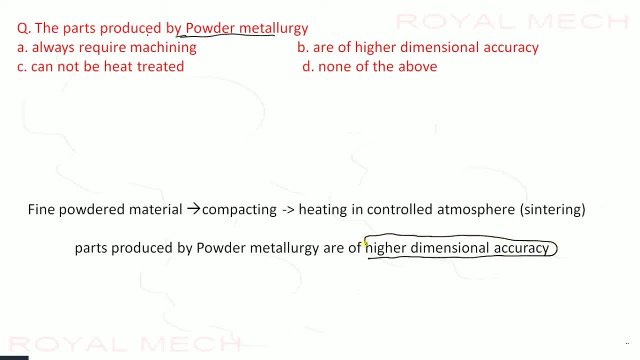 Just by production itself we can obtain the higher dimensional accuracy in powder metallurgy. And we know powder metallurgy process start with pine powder compacting, heating in controlled atmosphere or sintering. Therefore, option D is correct. Therefore, option B is correct option. 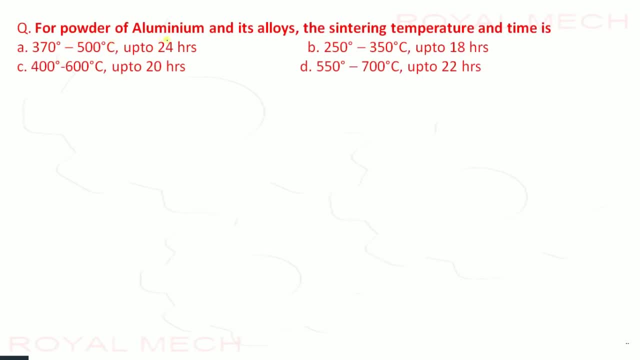 Powder of aluminium and its alloys, the sintering temperature and its time is. So we have to answer here. powder of aluminium and its alloys. sintering temperature: 370 to 500 degrees, That is the time. So So how much? 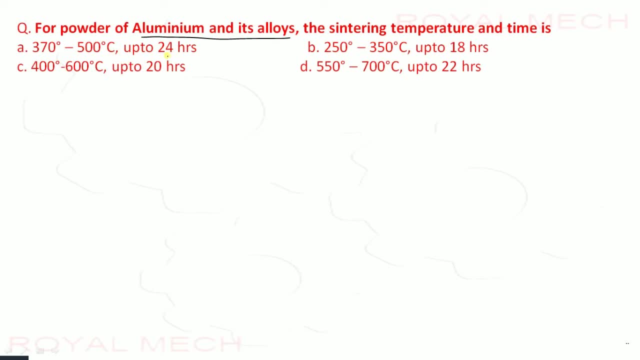 500 degrees. So how much degrees Celsius up to 24 hours: 250 to 350 degrees Celsius. up to 18 hours: 600 to sorry. 400 to 600 degrees Celsius. up to 20 hours: 550 degrees Celsius to 700. 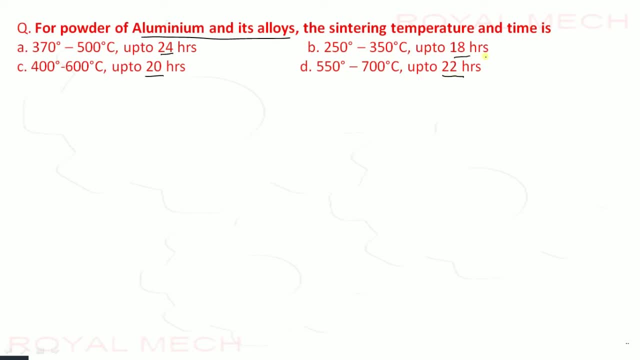 degrees Celsius up to 22 hours. so for aluminium, it and its alloys, the sintering temperature is 370 to 500 degrees Celsius up to 24 hours. that is option a is correct option. the factors influencing shrinkage during sintering include particle size, pressure, used sintering temperature and. 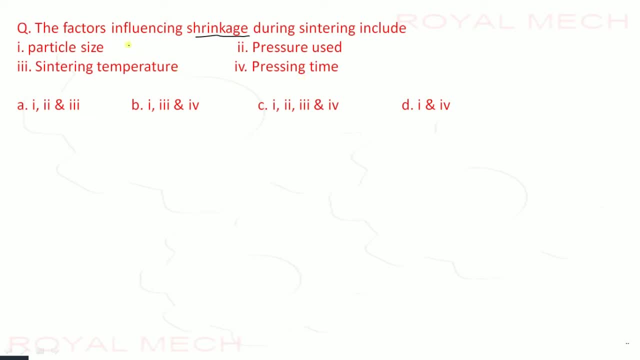 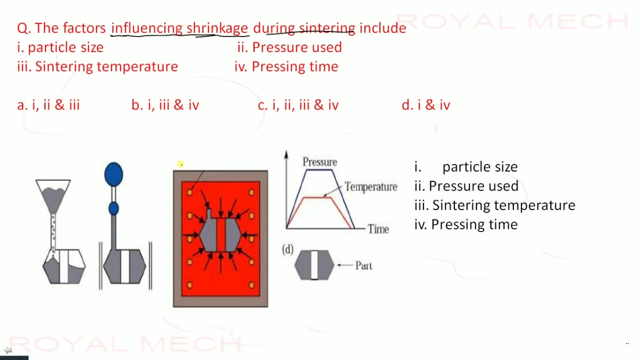 pressing time. so we need to answer which of the factors influence the shrinkage during sintering process. so when we see the sintering process, first of all powder is poured in a required shape and then it is heated, plus pressurized for some particular time that we can see here in the crop. 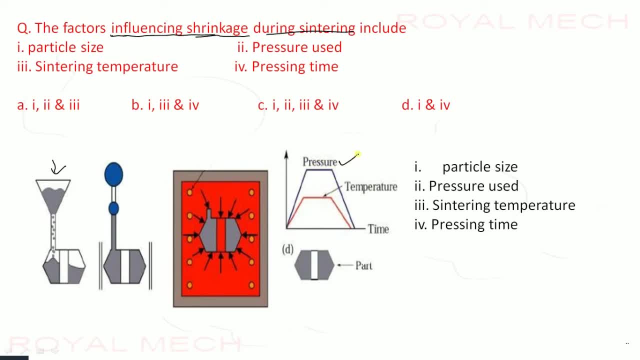 there is some pressure, there is some increase in temperature and it is been carried for a certain time. So shrinkage is been influenced by particle size, pressure used and sintering temperature and pressing time. that is how long we are going to press it. therefore, option C is correct option. 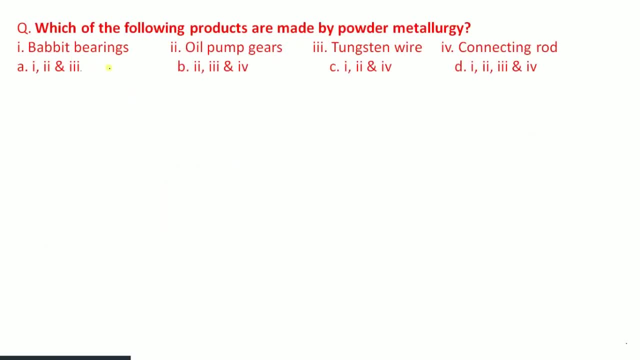 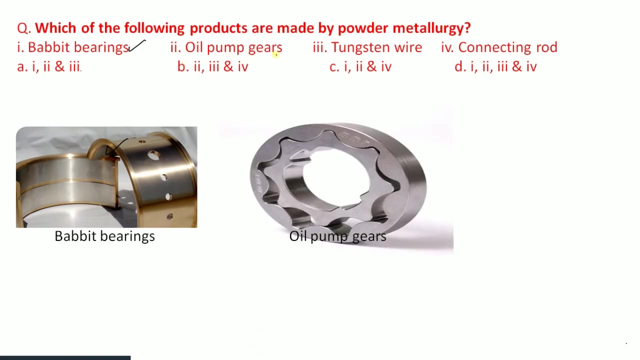 Which of the factors is correct? which of the selling products are made by powder metallurgy, Babbit bearing. so Babbit bearing are made by powder metallurgy. that is correct. Oil pumping gears: we can see here in the picture the oil pump gears are made. 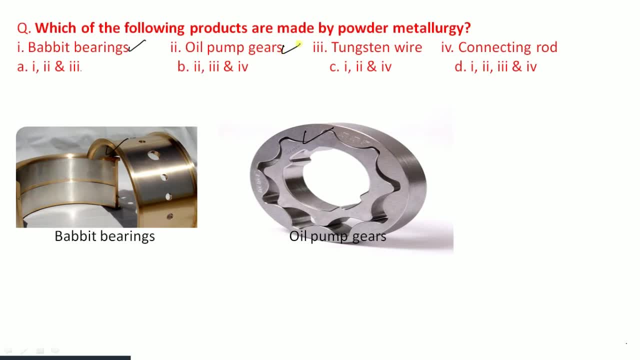 by powder metallurgy, that is correct. barrier, So air pump, bearing and justement- that is the final product- which are used in Kalis. the 순igung matter G, that is, callediries, is correct, is also correct tungsten wire, and this is also made by powder metallurgy. and 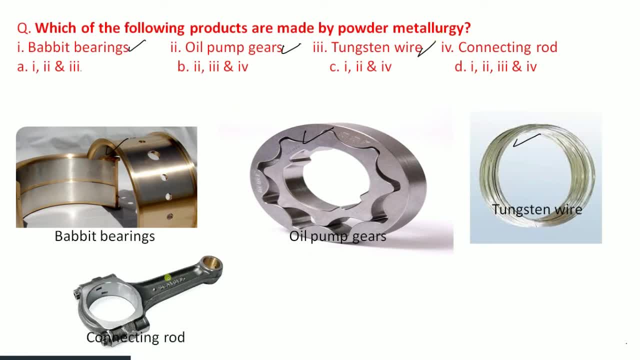 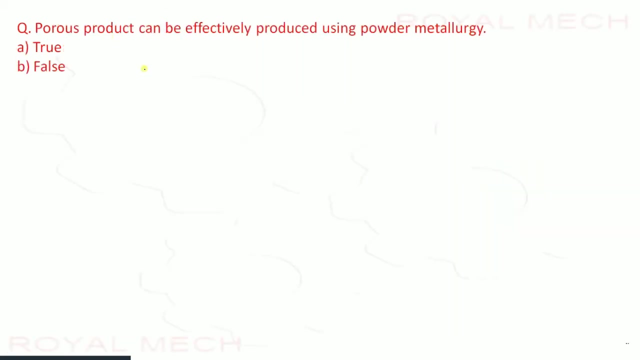 connecting rod. connecting rod is not made by powder metallurgy. therefore this is wrong. so here we can answer that one, two and three are made by powder metallurgy. that is option is correct option. porous product can be effectively produced using powder metallurgy, true or false? so powder metallurgy is best. 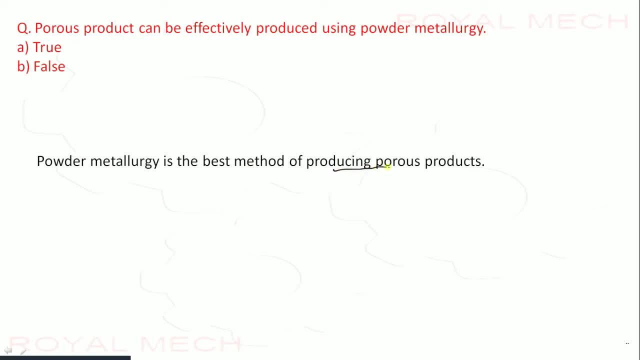 method for producing porous. porous products. that means this statement is correct. true dimensional accuracy in powder metallurgy is high, medium, low. none of the mentioned in product of powder metallurgy. it has high dimensional accuracy. therefore, option is correct option. range of particle size in powder to be used for powder metallurgy in microns should vary from: 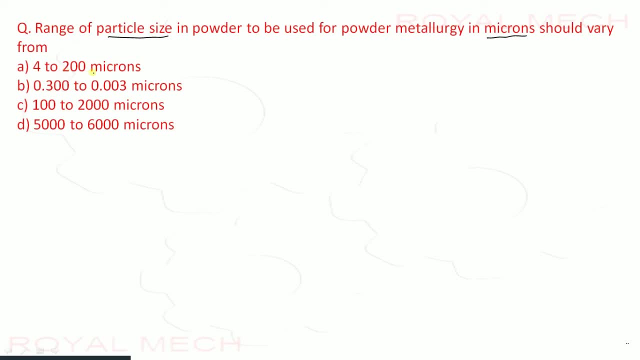 four to two hundred microns, 0.300 to 0.003 microns, hundred to two thousand microns, five thousand to six thousand microns. so the range of particle size in powder used for product metallurgy should vary from four microns to 200 microns. that is option, is correct option. production of. 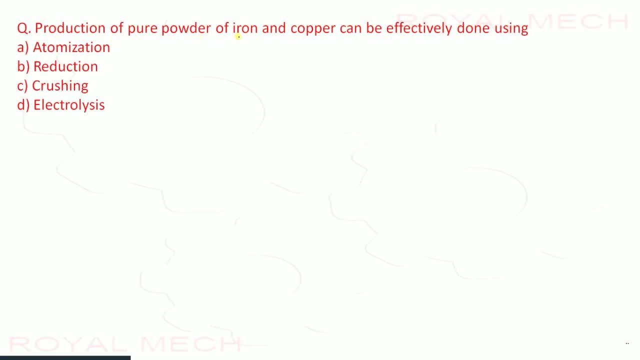 pure powder of iron and copper can be effectively done using atomization, reduction, crushing and electrolysis, So to produce iron and copper powder. electrolysis is the most effective process for formation of iron and copper powder. It uses two electrodes and electrolyte. 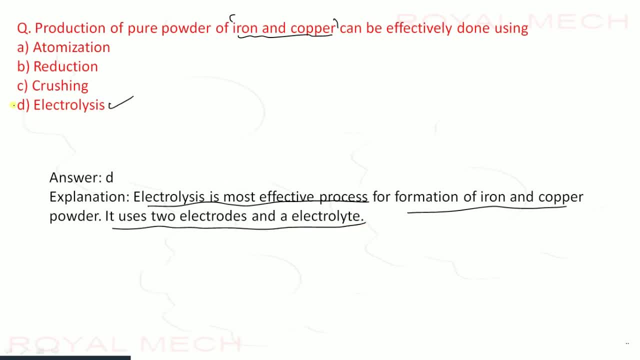 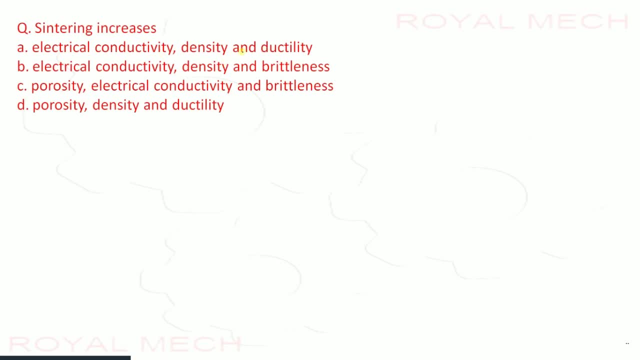 Therefore option D is correct. option Sintering increases electrical conductivity, density and ductility. Electrical conductivity, density and brittleness. Porosity. electrical conductivity and brittleness, Porosity, density and ductility. So here, sintering increases electrical conductivity, density and ductility. 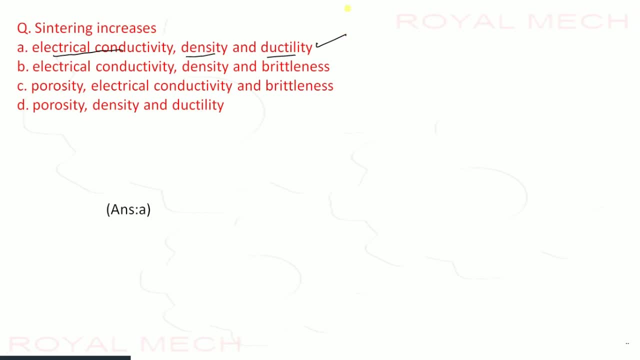 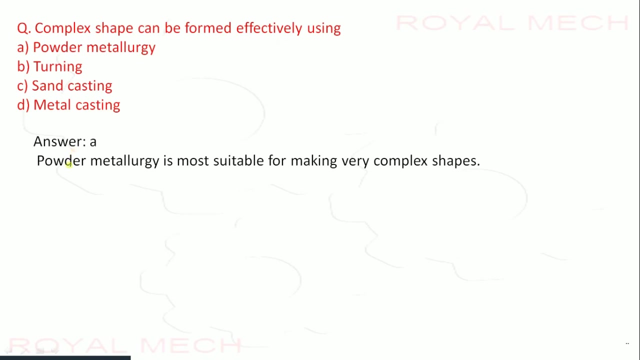 Therefore option A is correct option. Complex shape can be formed effectively using Powder metallurgy, Turning, Sand casting and metal casting. So the complex shapes can be produced by powder metallurgy, because powder metallurgy is most suitable for making very complex shapes. Therefore option A is correct option. 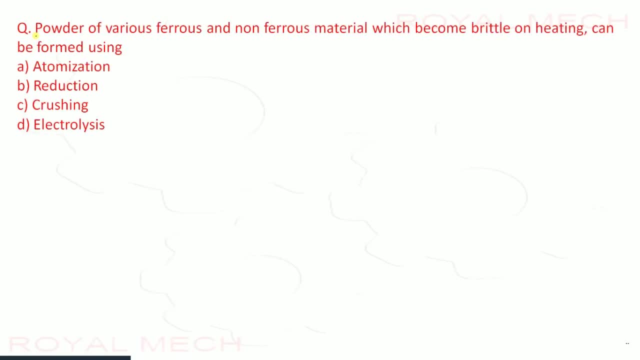 Powder of various paras and non paras materials Which become brittle on heating Can be formed using atomization, reduction, crushing and electrolysis. So for paras and non paras materials Which become brittle on heating, brittle on heating first, parasite and non-parasite materials are heated. 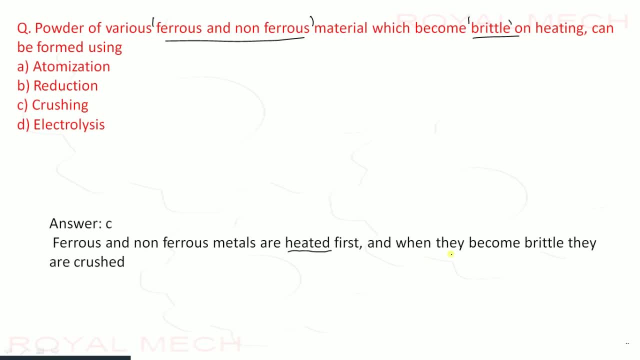 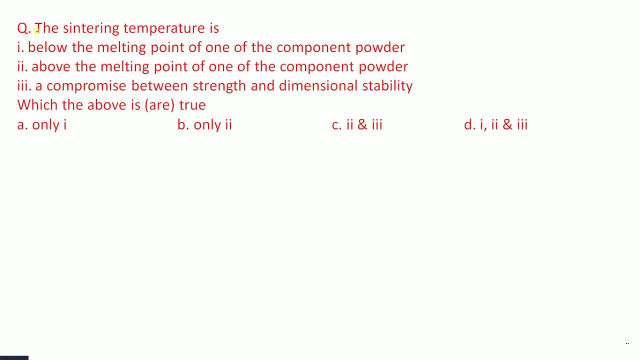 and when they become brittle they are going to crush it. therefore, it is nothing but the crushing. therefore, option C is correct option. the sintering temperature is below the melting point of one of the component powder. it is below the melting point and, in second option, above the melting point of. 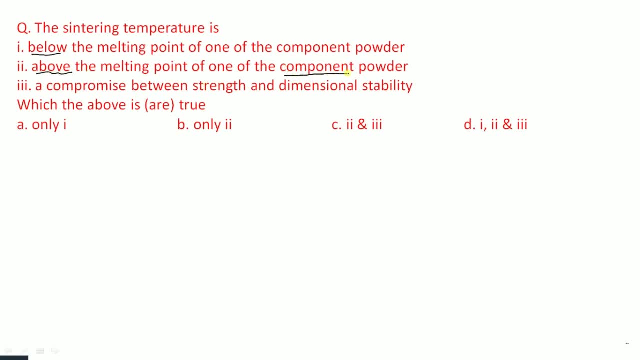 one of the component powder, a compromissive between strength and dimensional stability. so sintering temperature is above the melting point of one of the component of powder. that is, one component temperature is above its melting point and a compromise between strength and dimensional stability. therefore, option C is correct option.